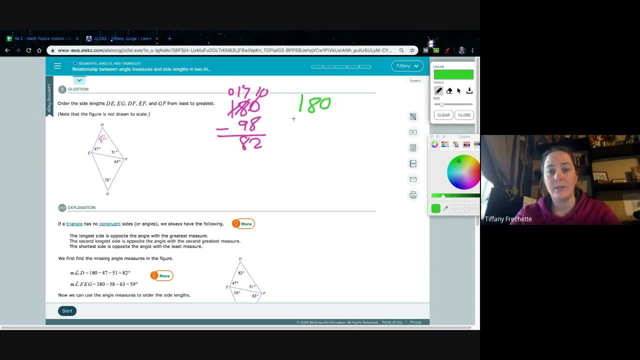 down here, So I know I have 180 degrees, because it's just another triangle. I'm going to add these two together, so I get 11 and 12.. I get 121. I'm going to subtract, so I get seven and then 12.. I'm going to subtract so I get seven and then 12.. The difference is 7, and 11.. So I all in turn have four angles, one below the other and two between them. All in turn are the angles I end up: atwheel base, seven and 12.. 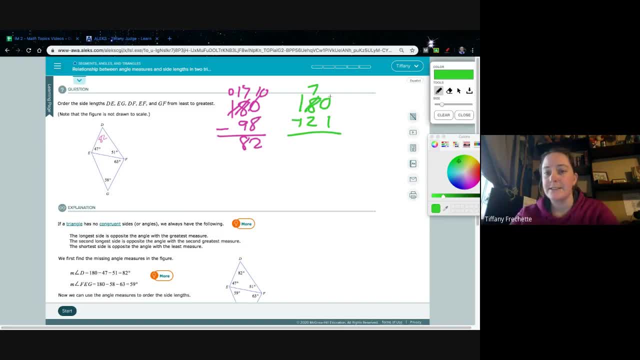 All in turn have four angles and I end up atwheel base 17 and 12. Quarter angle is equal to 18. кв. undivided queen by bayou. So I get seven, one, nine and five. So I get 59 degrees in here like this: 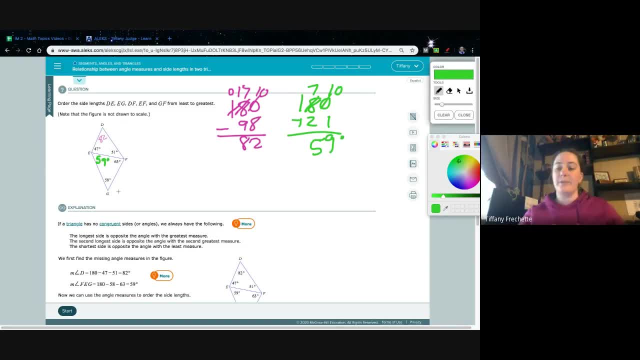 And I should have made my pencil a little bit smaller on that one, just so that it fit a little better. but that's all right. All right, so we filled this in. So now we wanna start going across and figuring out the side lengths. 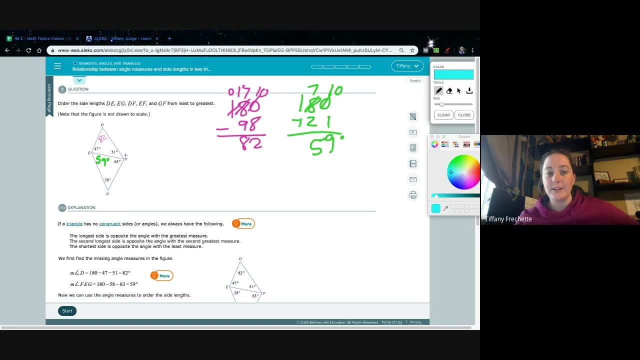 that are the greatest and the smallest. They want us to do, from least to greatest. So first let's focus on the triangle on the top. So the smallest angle on the top is 47, so I'm gonna go across. So I know DF is the smallest side. 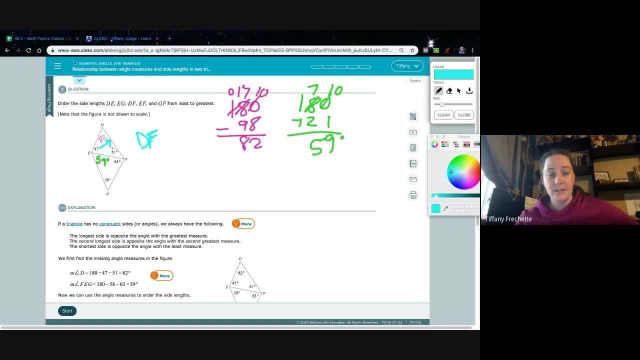 DF is the smallest side, The next greatest or the second greatest measure, or least measure, I guess, since we're starting from smallest, the second least measure would be 51, and I'm gonna go across and I'm gonna go to DE. 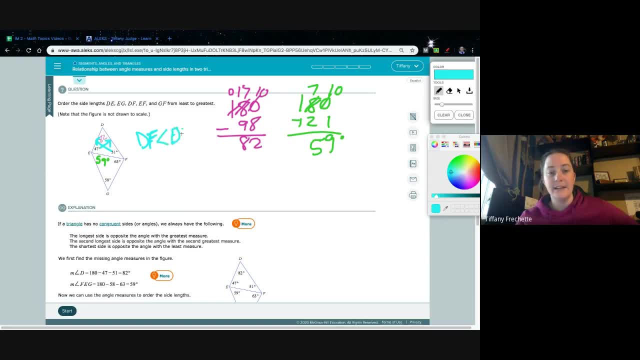 So DF is smaller or less than DE, Which is less than this last measure, which 82 is the biggest one. So I'm gonna go across here. So I have EF like that. So this is my top triangle. I also have a bottom triangle. 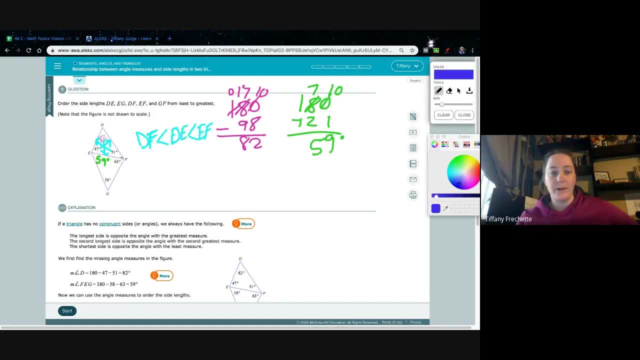 Let my bottom triangle here put it in dark blue, why not? All right. so then my smallest one for the bottom triangle is GF And that's smaller than 58.. Oh, nope, I did that wrong. 58 would be the smallest one, wouldn't it? 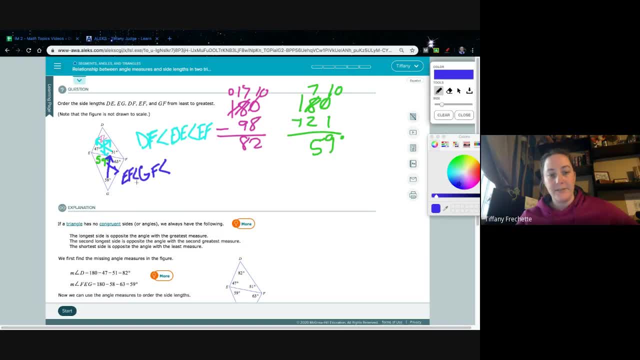 So EF- I'm gonna stick this on the front. EF is actually the smallest, GF is bigger than EF is 59 is just bigger than 58.. Just wasn't I mixed up my numbers there. And then 63 is pointing at the smallest one. 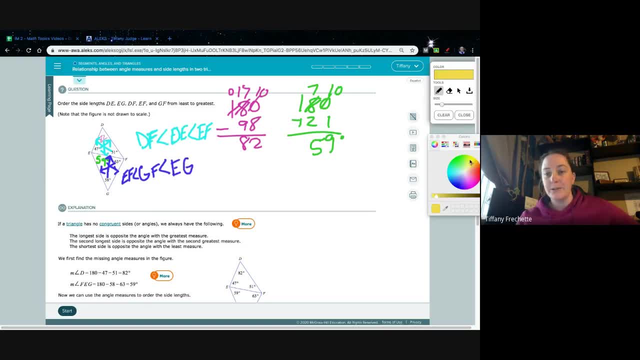 So EG, So we wanna do here- and I'm gonna kind of pick an orangey color- We wanna put these together. So we know EF is larger than these two, but EF is smaller than these two. So this is actually going to be the middle. 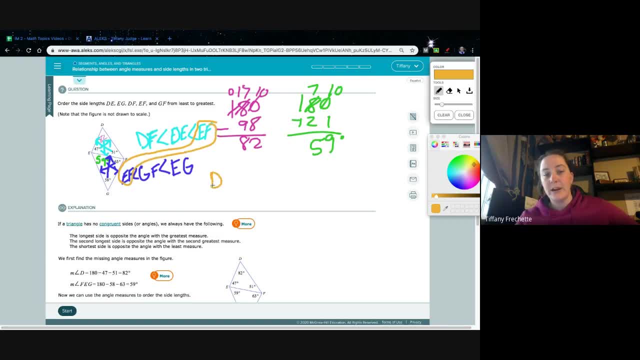 We're gonna stick these two together, So we're gonna rewrite it all as one. So DF is less than DE, which is less than EF, And instead of writing EF again, I've already written it, So I'm just gonna continue. 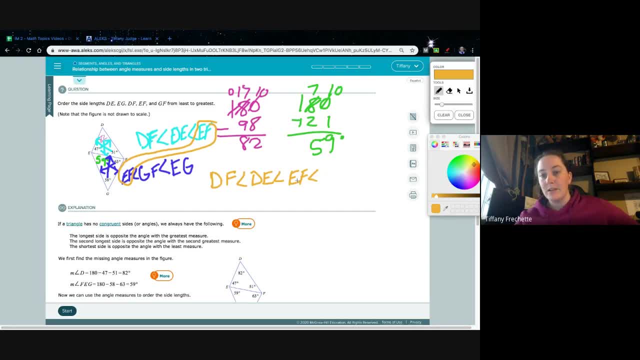 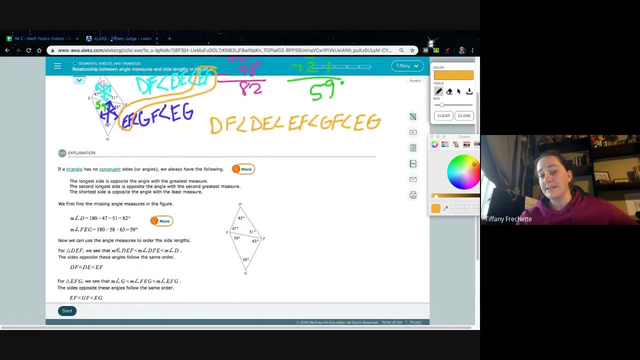 help if I was paying attention when I was writing. I'm just gonna continue writing this GF and then EG like this. So if we scroll down to the bottom here, that's exactly what they have. They have this nice long list. So on the next page we're gonna actually get started. 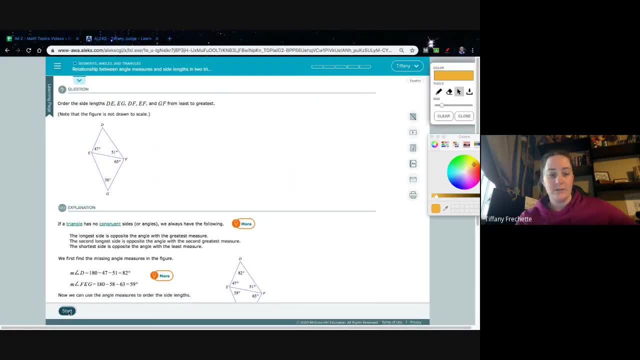 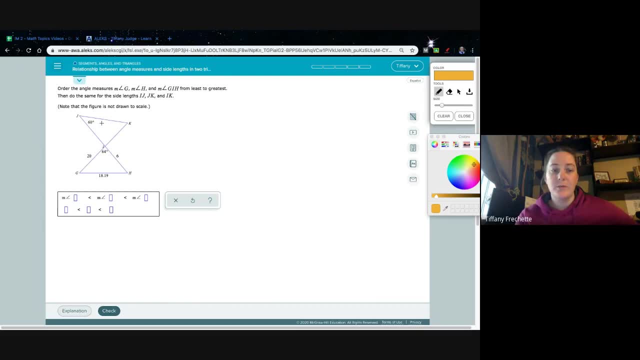 Listen, let's clear this out and let's go ahead and start. So okay. So first we need to, we need to write this down, First we need to start filling in some amounts based on what we've got here. They want us to do. angles. 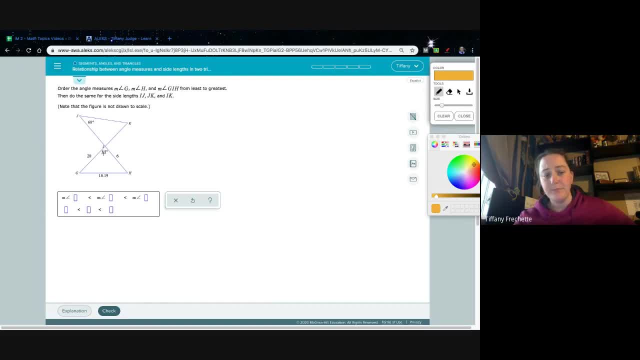 So they gave us a couple of angles here, And then they want us to do the rest of the angles. Let's see, Oh nope, I'm lying. They only want us to do angles for one and then do the same thing for the sides. 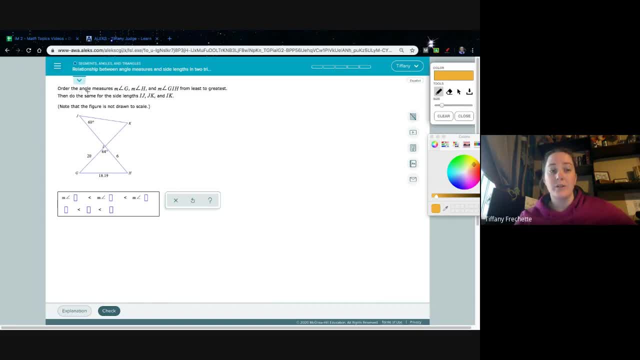 for the other triangle. So for order, the angles, angle measures, angle G, angle H and angle GIH. So this one, they want us to put these in least to greatest first, And then they want us to do lines IJ. 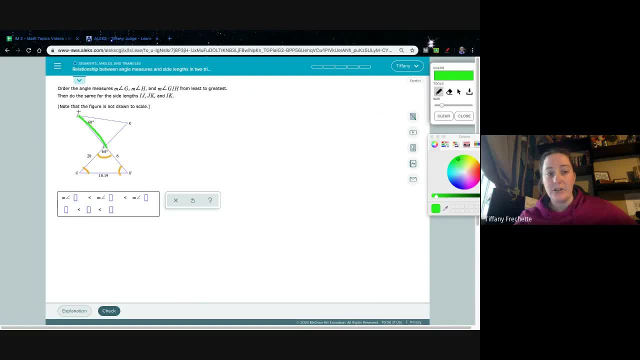 So this one up here: IJ, JK and IK. They want us to put these angles in order from least to greatest, and then the sides in order from least to greatest. So let's go ahead and look at the angles first, Just like side, or the side lengths that are across. 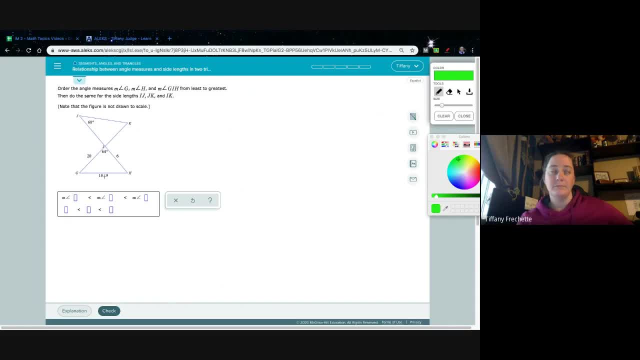 from the- I'm saying that funny- the triangle inequality theorem. geez, Louise, I'm saying this really funny. I'm sorry It works both ways. For some reason I can't get my words out there, but the greatest side is across from the greatest side. 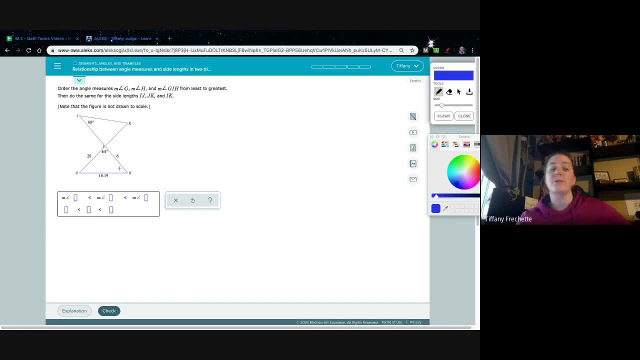 The greatest angle is across from the greatest side, So I can go back and forth either way. So I'm gonna go the smallest side because it wants least. So six is smaller than 18.19 and 20.. So my smallest angle is G. 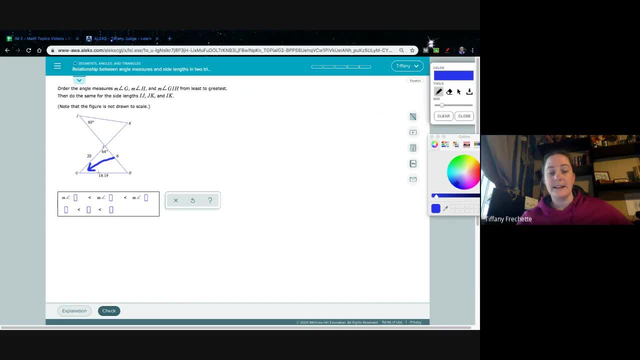 I'm gonna write G here in just a moment. 18 is the next smallest or next least, So I'm gonna write angle GIH. I don't wanna write 64, they don't want the degrees And I can't write I because I could be here. 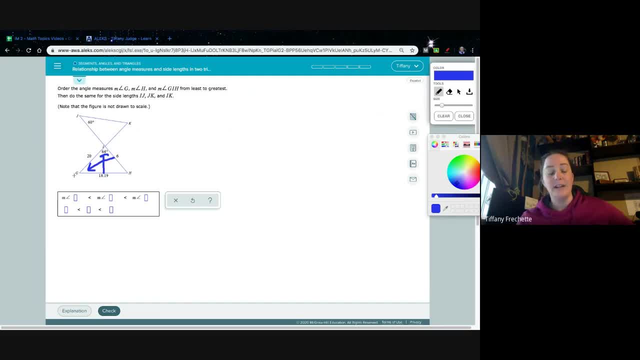 or it could be up here on the top. So I have to use three letters to identify that angle. I have to use the two ends of the vertices here, which are kind of the rays coming off, and then the vertex is in the middle. 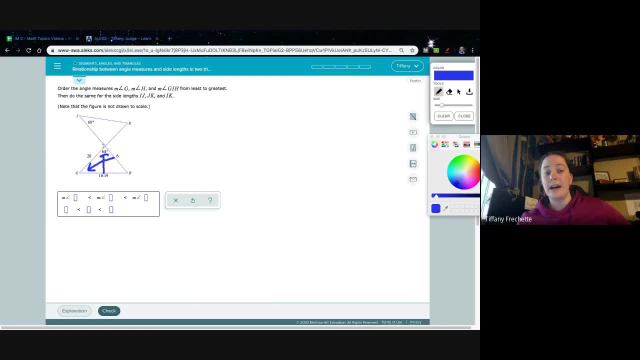 So the vertex in the middle tells me which angle it is. So I want I in the middle, but then I need to describe it GIH, And I'm gonna go ahead and type these in. So I have G and then I have GIH. 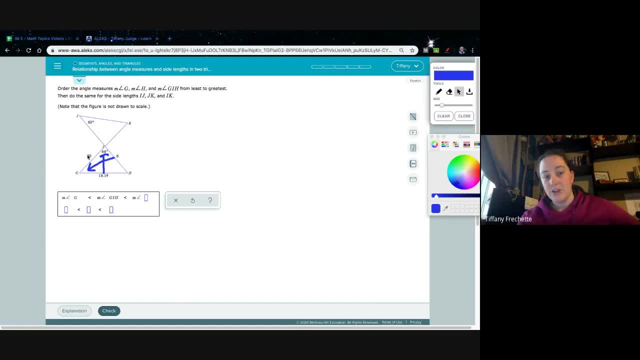 And then the next one is going to be H here, because 20 is across from H, All right, so I'm gonna clear that out real quick, and then we're gonna look at the side lengths. So one thing we do need to remember from this one: 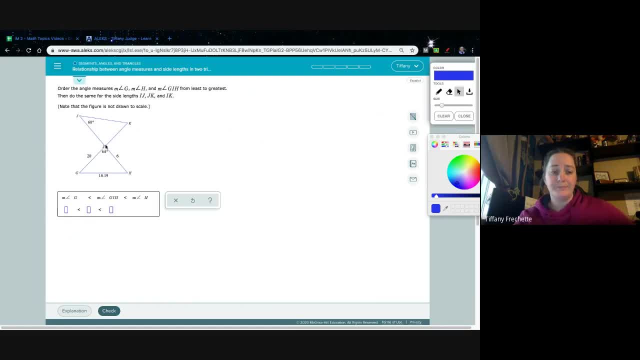 and this is back kind of from I am one- is that we need- not only do we need- to know all three angles, and we're gonna put the sides in order, but we only are given one angle. So if I can go across the vertex like this: 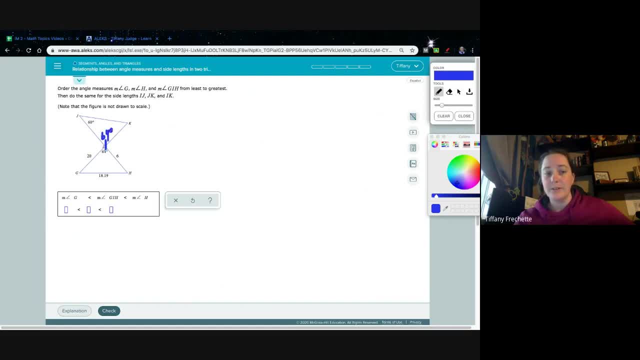 we call it a vertical angle And vertical angles are always congruent. So if I have, this side is 64, this side is also 64. So now I have two angles, so I can subtract from 180, because, remember, they always up to 180. 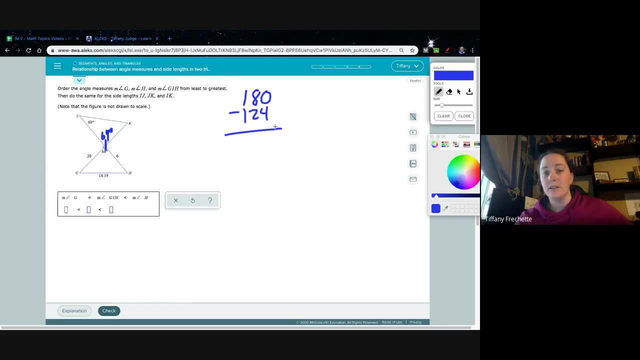 So I have 60 plus 64, that gives me 124.. I'm just gonna subtract Doop-de-doop-de-doo, Mixing up my words earlier. That's what happens when you do too many of these at one time. 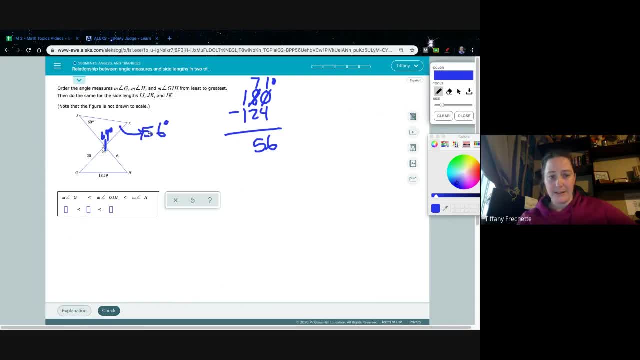 All right, so 56 degrees it goes in here. So now I just wanna start putting them in order. So 56 is my smallest, So I wanna go across from 56, and I get IJ, That's my smallest. 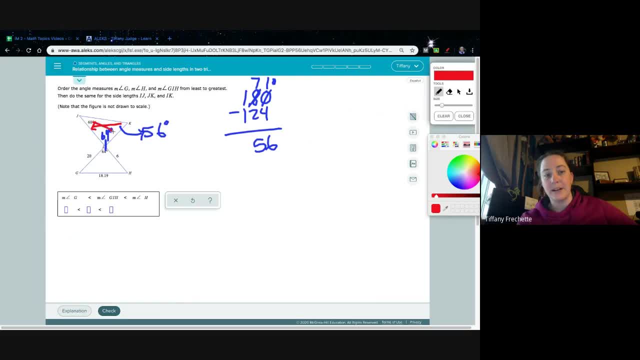 Then I'm gonna go to 60, because that's my next one in line, So I'm gonna have IK. So let's go ahead and type this in so we don't get ourselves mixed up. So IJ goes first. First, then IK. 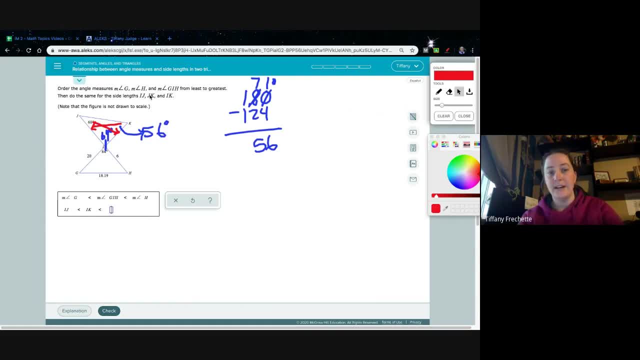 And the only one that's left in our list here, because IJ and IK would be JK And if we test that, 64 is the biggest. If I go across, there's JK. All right, check and we're good. 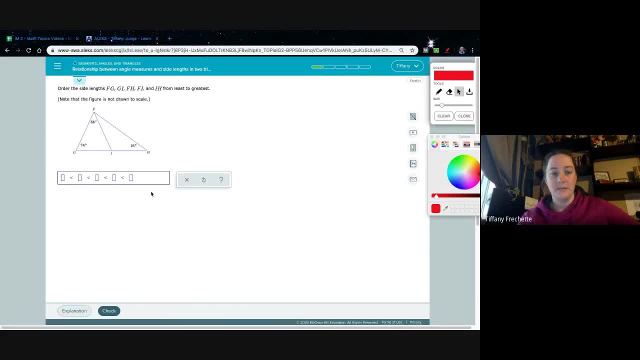 All right, so let's clear that Next. Okay, so this one. they want us to put all the lengths in order this time, So we're only looking at angles. So first let's look at this, This triangle on the left. 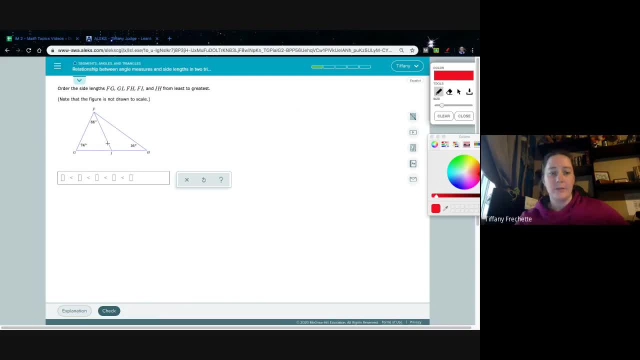 So we wanna know what is this length right here, Or not length, sorry. What is this angle? So again, we have 180, and we wanna subtract what we've already used here. So if I add I get 10 and 14.. 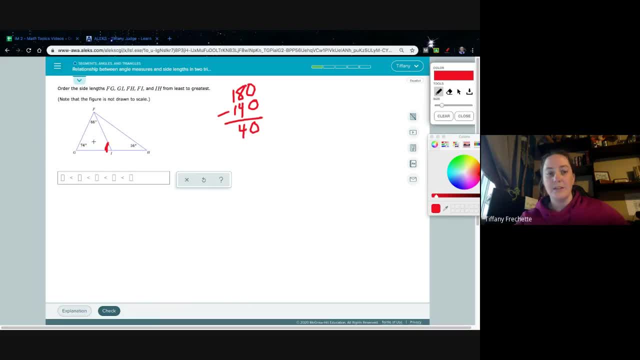 So I only have 40 left over when I subtract, So this has to be 40.. So now let's go ahead and put them in order. So 40 is the smallest, So I'm gonna go here. So GF is the smallest. 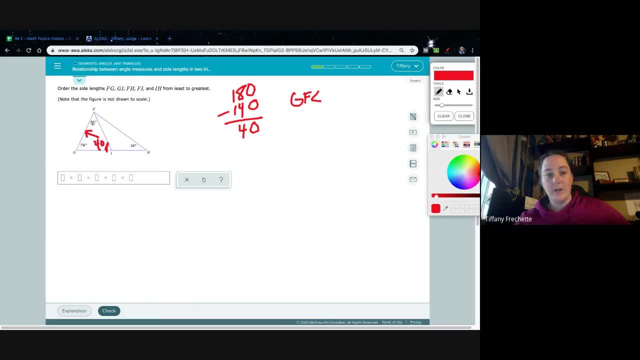 The next one would be across from 66 here, So it'd be GI, And then the biggest one here is across from the 74. So it's right here. So this is FI All right, so now I've put these ones in order. 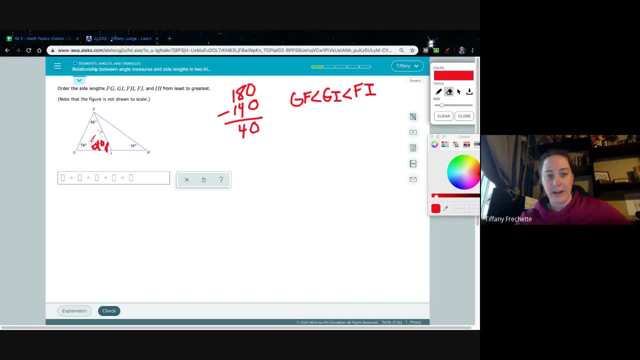 And I'm going to erase a bit here because it's a little too much to look at for the next triangle. So I'll put a little bit back there. But Look, I'm gonna put the 40 degrees back, All right? 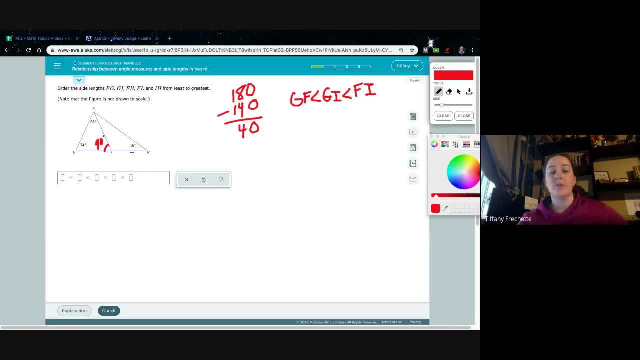 So now I need to figure out this triangle and I need to put them in order least to greatest, but I only have one angle. Well, if we remember again back from I am one. a linear pair means that angles on: 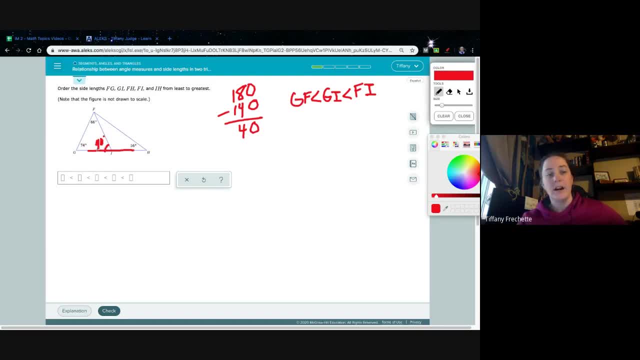 they are two angles on the same line, or at least two angles on the same line, And if they're on a line, a line always equals 180 degrees. We really like that 180.. So I'm gonna change this to blue. 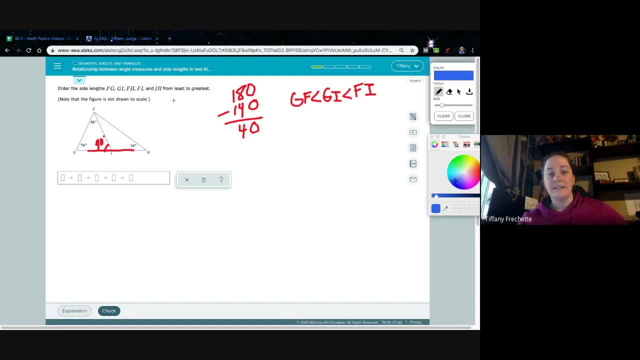 If I know this is 180, then I can say, well, the whole thing's 180.. I'm using 40 degrees, So this angle here must be 140.. I'm gonna write that really bad, This one's 140 in here. 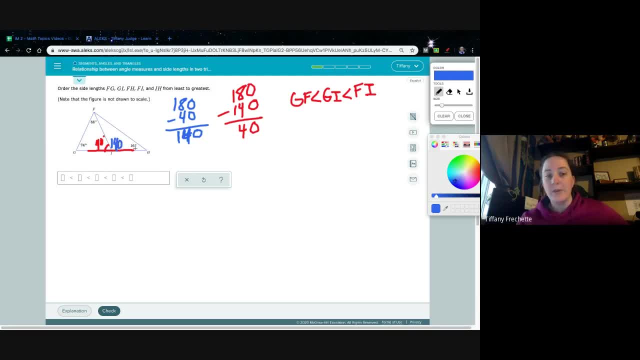 Boom. All right, So now we have 140.. We have 16.. We need- We need to figure out what this one is up here. So again, we go back to our 180.. It's a triangle. All together they have to add up to 180. 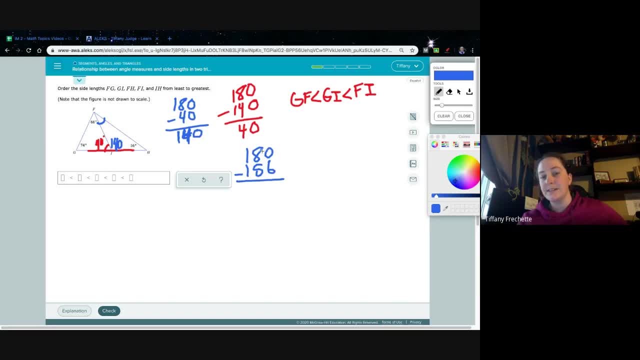 So I know 140 plus 16, that gets me 156.. I'm going to subtract and I get 24.. All right, So 24 degrees in this one, All right. 24 is definitely Or no, 24 is not the smallest. 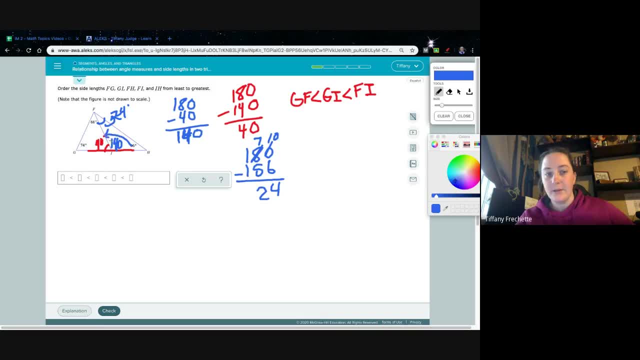 16.. 16 is the smallest, So we're gonna go across and I'm kind of going around the 140 there. So FI is the smallest in the right triangle And the next one would be the 24. So I'm gonna go across here. 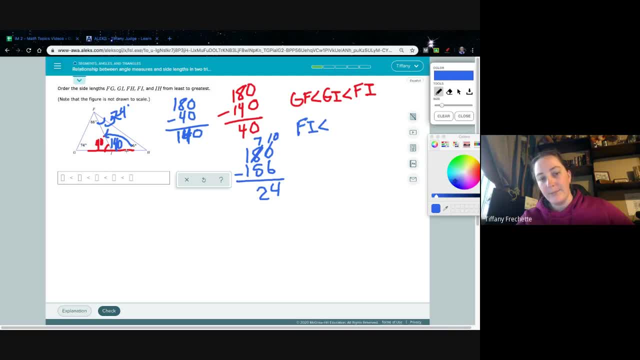 and instead of drawing over these numbers, I'm just gonna kind of let my cursor follow. So now I have IH, And the biggest one would be across from the 140 here. So that would be the FH. All right, Nope H. 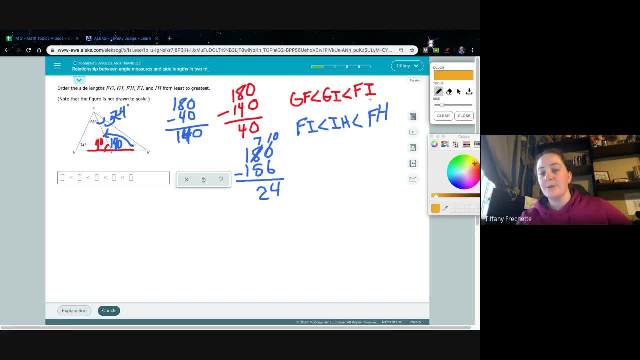 All right, Now I'll pick an orange, just like I did before. So what we're looking for is one that's repeated. So the only thing that's repeated is FI, And, honestly, it should always be the end of one and the beginning of the other. 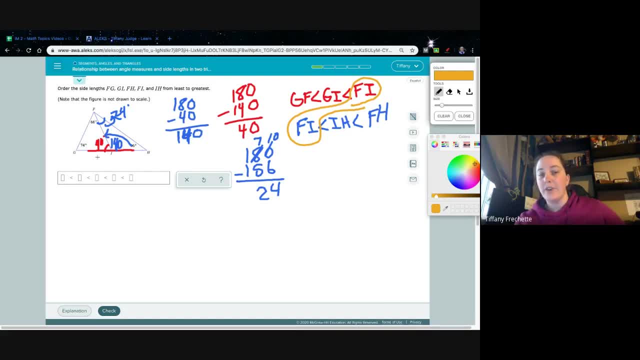 That's how it should always end up. Depends on which triangle you did first. So in this case we had to do the left triangle first, because I have to find the 40 to find the 140. And then I use the 140 to find the 140.. 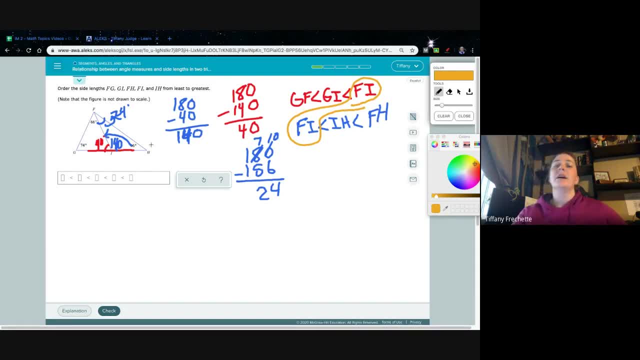 to find the 24.. So I kind of have to go in that order. We didn't necessarily have to put them in order. first, though, I could have found all my amounts, and then I could have done this blue list first and then the red list. I just decided to make the list as I went, So it's just one of 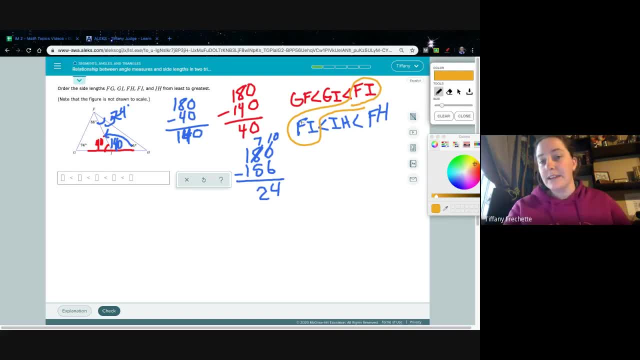 those things. Just make sure it's ones at the beginning, ones at the end, and then you want to just put them in order. So I know these are smaller than Fi. These are larger than Fi. So as I rewrite this, I just want to make sure Fi is in the middle, like this: 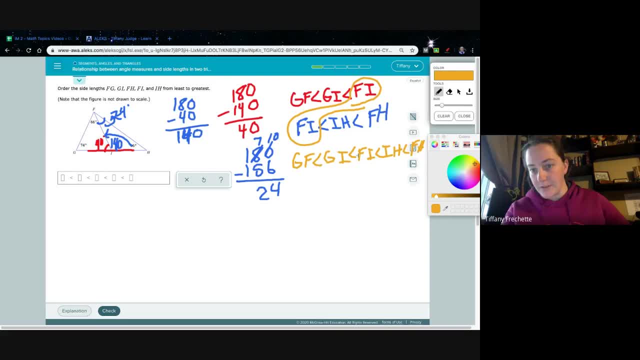 And I'm going to end up writing my tools here. So here's Fi. Here are the two that are smaller. Here are the two that are bigger. So that's the basic idea, So we just need to type it in, So I. 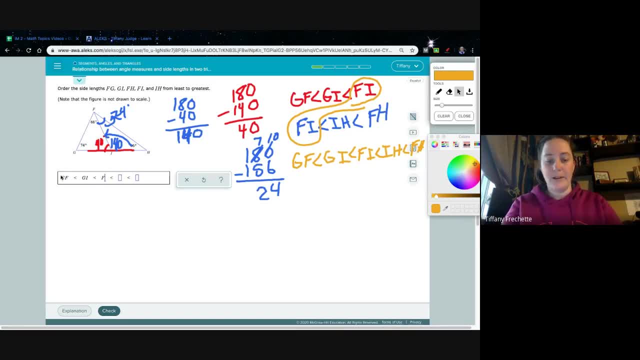 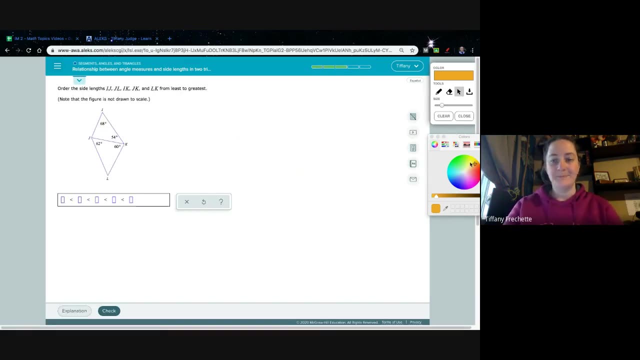 didn't necessarily need to write it out each time like that, But I'm going to show you before I typed it in here. Okay, Check, Yay, All right, Clear And one more Next. All right, Let's go to kind of a pretty green here, All right, So again. 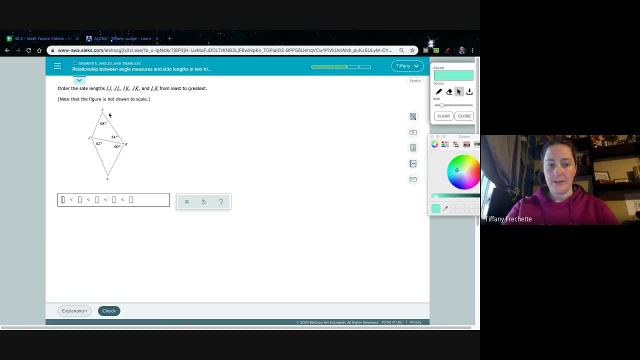 they want us to put all the lengths in order from least to greatest. So this one's a lot like that first one we started out with on the example. So we need to find my pen on, We need to find this length here. I keep saying length, this angle here. So we have 180 and we want to subtract what. 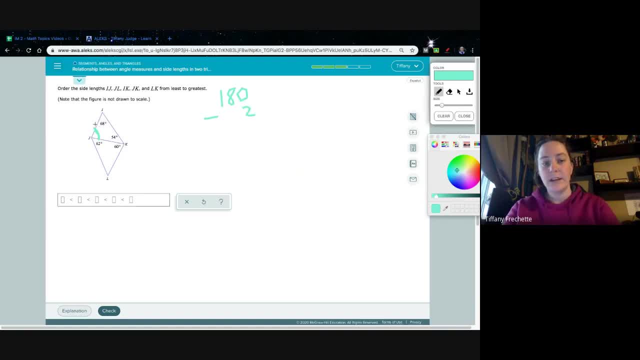 we have here. So let's see, That's 12 and 11, 12 again. All right, So we're going to subtract 7, 10,, 8, 58.. So this is 58 in here, All right, And then I'm going to go ahead and put them in order, since I'm already. 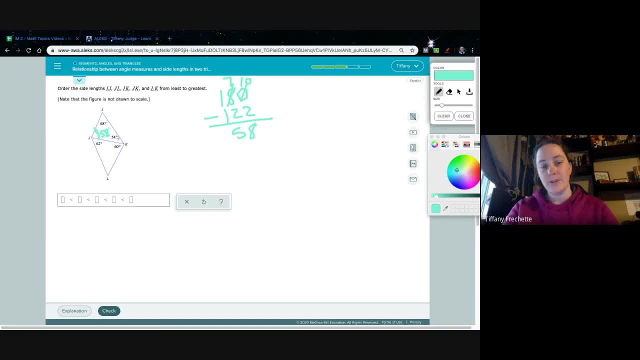 starting. So again, it's kind of a little too scrunched here to actually do arrows. But 54, I'm going to go across. So that would be IJ, And I'm just saying IJ because that's the way they put it. 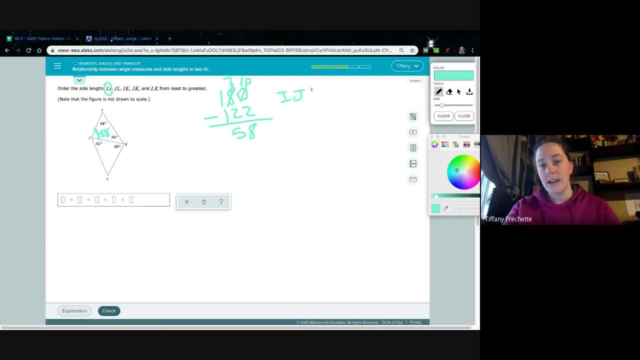 up here is IJ. IJ is less than I'm going to go to the 58 because I'm just going in order. So I go over here and I have IK And that's smaller than across from 68, which is my biggest one, which would be JK And I 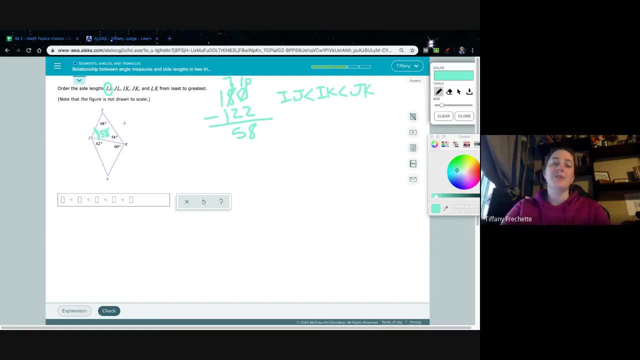 don't necessarily think it's not going to mark you wrong if you put them out of order, Like if you put them, if you put these out of order, to mark you wrong. what I mean is if you switch it, if you said JI. 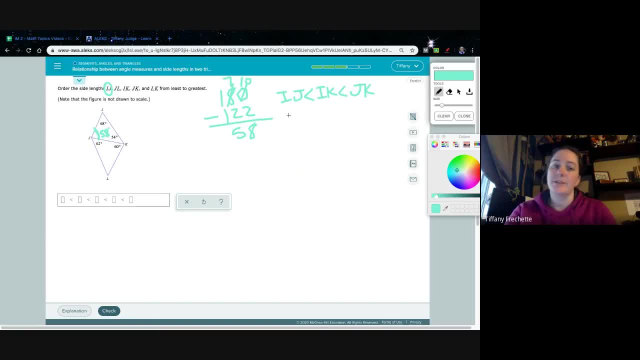 Or KI Alex isn't that picky where it's going to mark you wrong in that way. All right, Go down here. We haven't used a purple, Let's use purple. So now we need to find this angle here. So again going. 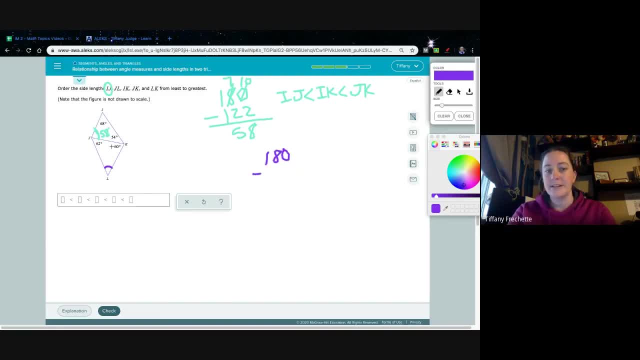 back to my 180 and I'm going to subtract what I'm already using here: 60 plus 62 is 122.. And I'm just going to subtract, I get 58.. I get 58 in here also. It's just different numbers, but we end up with 58 left over for each one. So it's: we ended up 122 for both of. 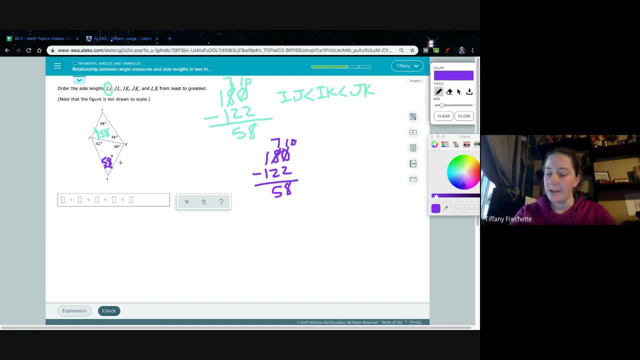 these added together, But it's just still slightly different triangles. All right, So 58 is our smallest. I'm going to go across and I have. JK is less than JL And I think they did- yep, they did do JL. 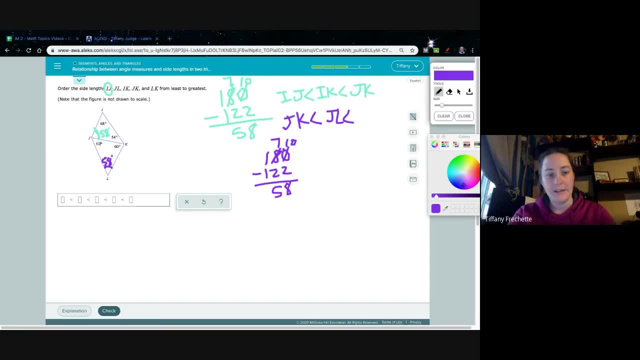 Sorry, I was looking at the list up here And then 62 is the biggest one. So this would be LK And I'm putting it in the same order that they're listing it in. But, like I said, it shouldn't matter if you put KL or LK. So if we notice again, we have JK at the end and JK at the beginning.